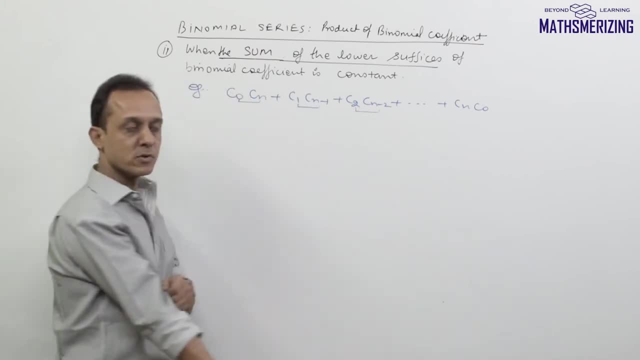 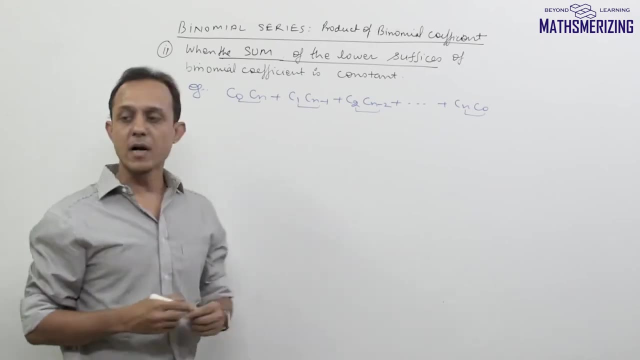 1 plus n minus 1, again n. 2 plus n minus 2, again n, and then it continues up to n plus 0, which again is simply n. Now, in this case again, we will start the expansion of 1 plus x to the power n. 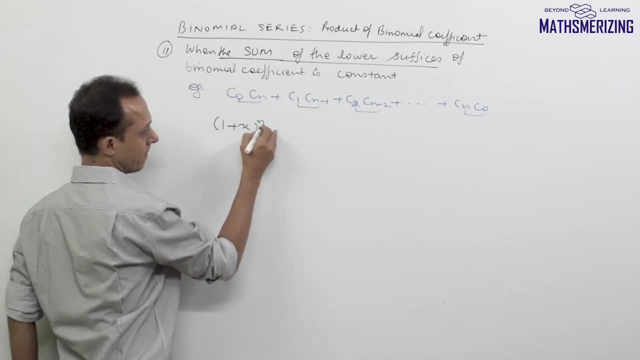 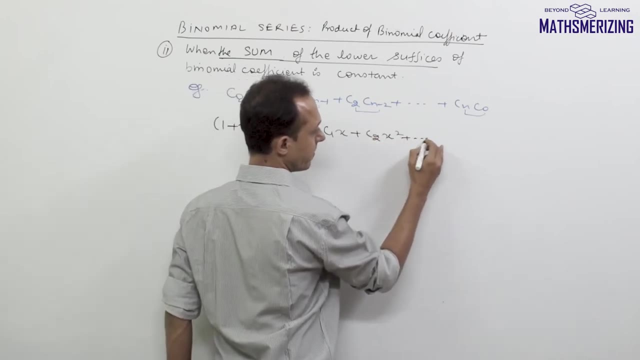 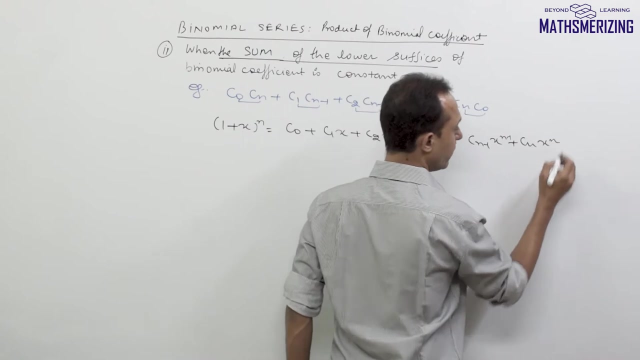 so simply it will be c 0 plus c 1 x, c 2 x square, and then c? n minus 1 x to the power n, minus 1 plus c n into x to the power n, and again I'll take the expansion of 1 plus x to the power n. 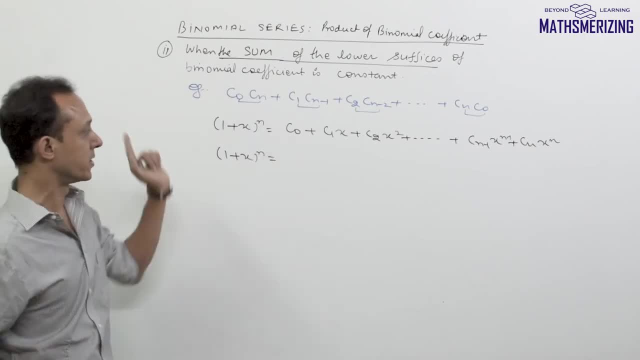 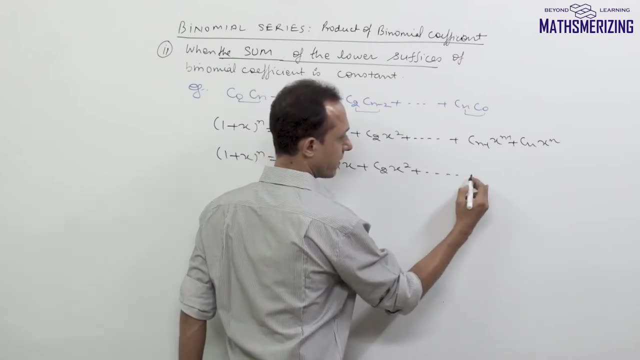 So in this case I need not reverse the series, because already sum is constant, right? so again I'll write c 0 plus c 1 x plus c 2 x, square, c n minus 1, x to the power, n minus 1, and then c? n into. 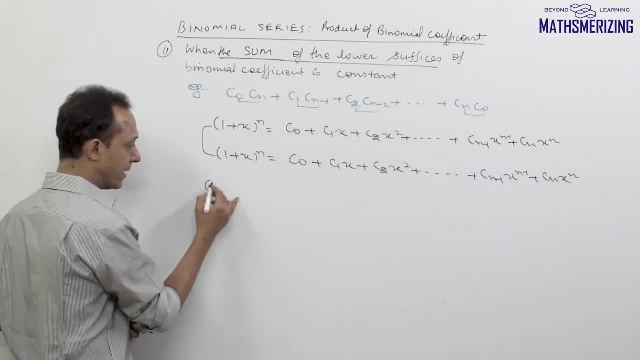 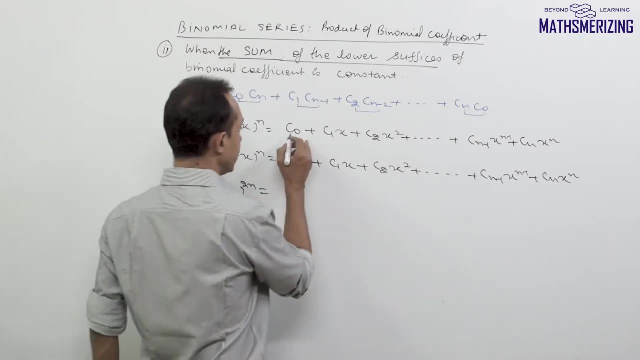 x to the power n. Now I'll start multiplying them. so if I'll multiply it I'll get 1 plus x to the power 2 n, and then I need to multiply this c 0 with c n, so I won't bother about other terms. 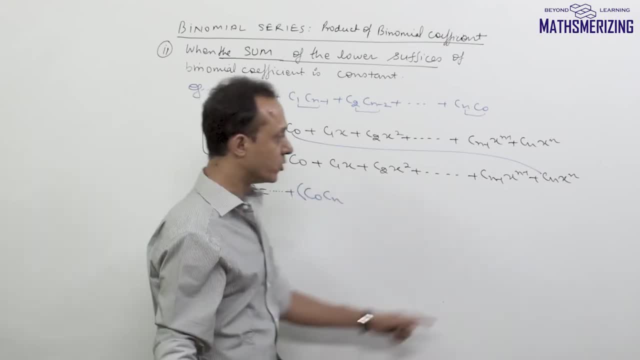 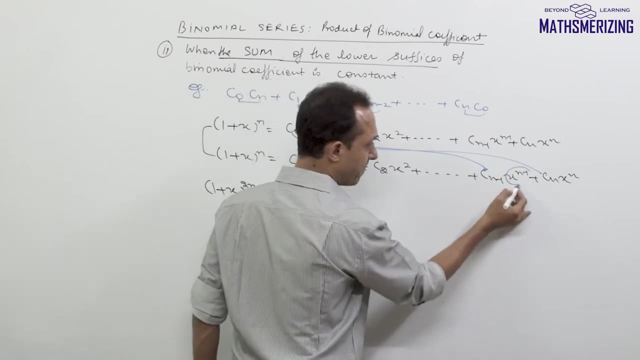 so when I'll multiply c 0 with c n, I'll get x to the power n. and then I'll multiply c 0 with c n minus 1, so it is x to the power 1, and it is x to the power n minus 1, so again it is x to the power. 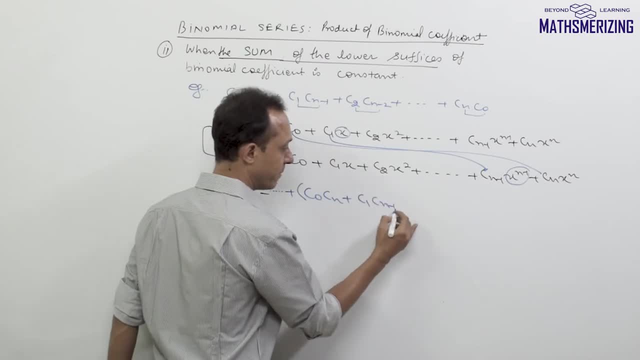 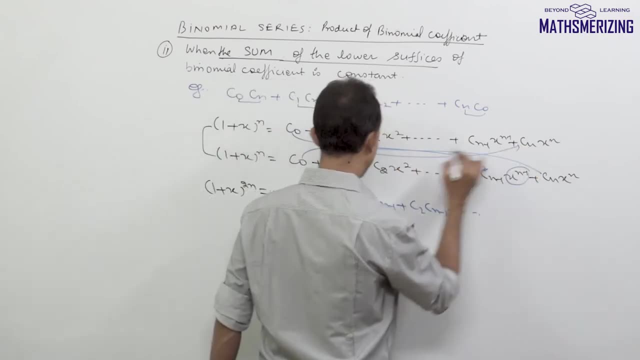 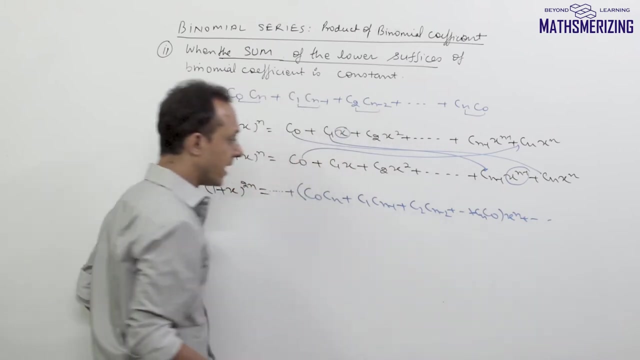 n. so plus c 1 into c n minus 1. so again then c 2 into c n minus 2. so it'll continue. and finally c 0 into c n. again it'll come with coefficient of x to the power n. so that is if I have to find. 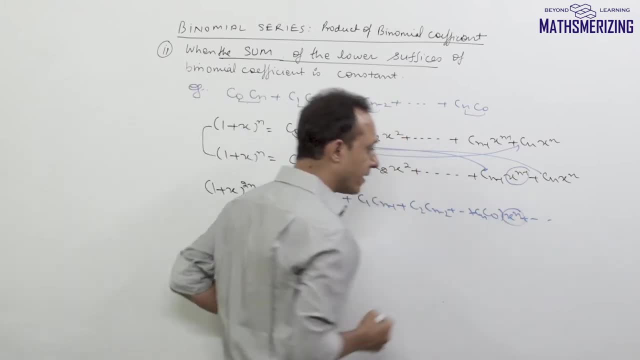 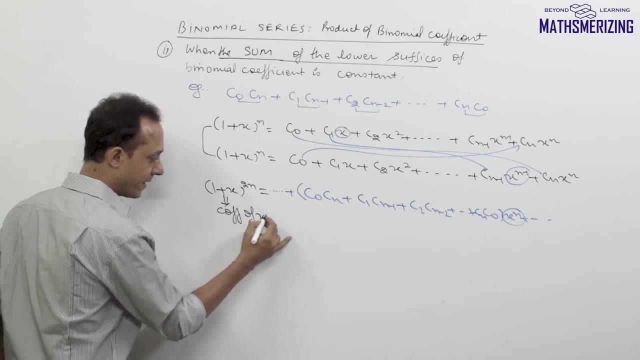 the sum of the series. then all I need to do is- I'll take the expansion of 1 plus c, 1 x square c- I just need to find coefficient of x to the power n on the left hand side. so I need to find coefficient of x to the power n. so what is the coefficient of x to the power n and 1 plus x to? 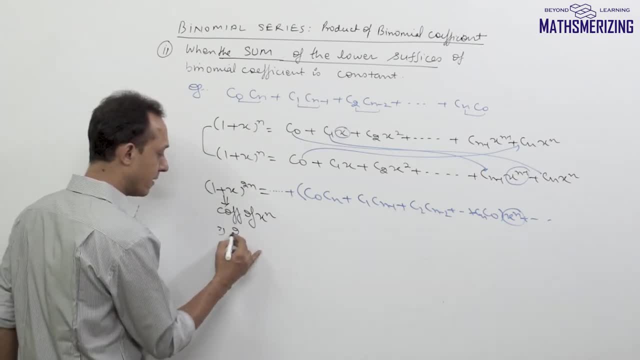 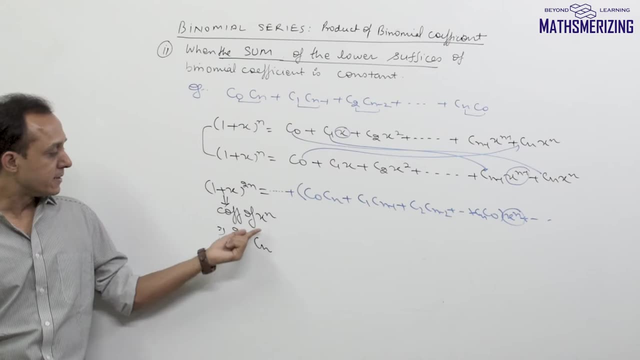 the power 2 n. so coefficient of x to the power n simply will be 2 n c n. so coefficient of x to the power r in 1 plus x to the power n is n, c, r. so that is 2 n c n. so that is the answer to this. 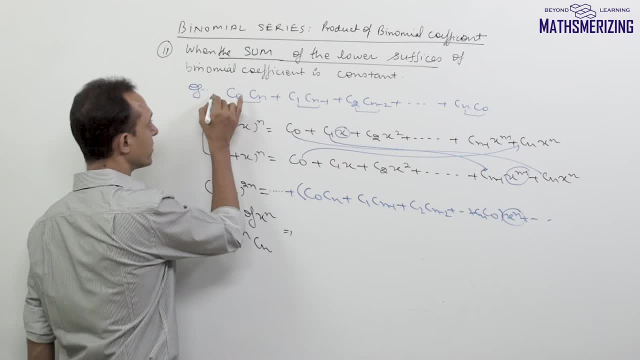 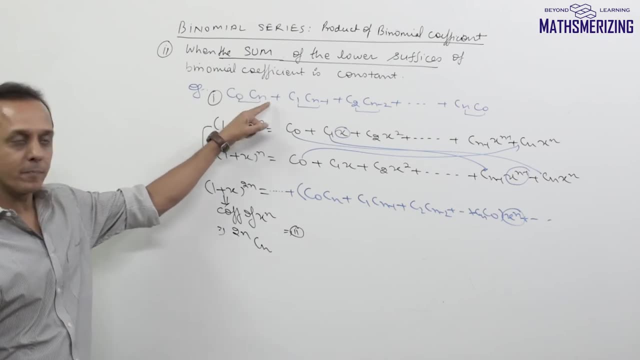 question and I can also write this result as nCr is same as nCn-R, So nCn will be nC0,, nCn-1 is nC1, nCn-2 is nC2.. So the same result. 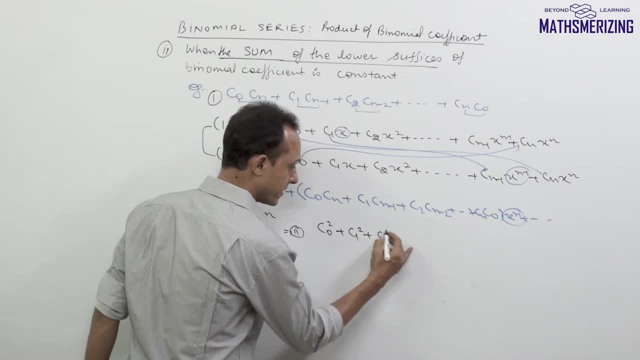 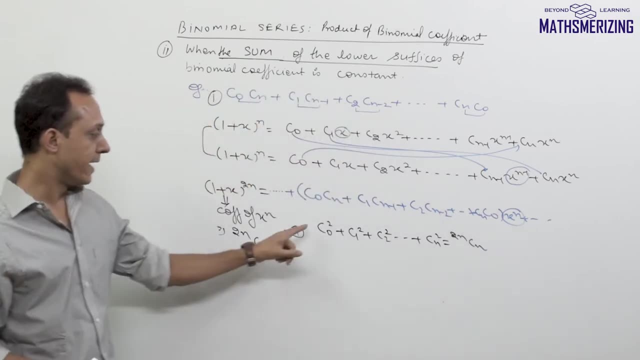 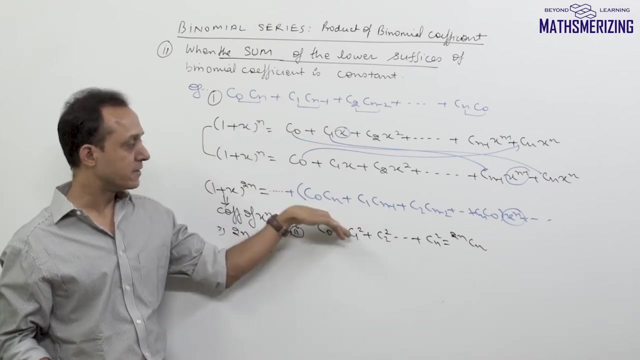 can be written as C0 square plus C1 square, plus C2 square and plus Cn square again will be 2nCn, which is again same as the case where the difference of suffix is constant. So this is the alternate expression of the same series. Let us consider another binomial series which 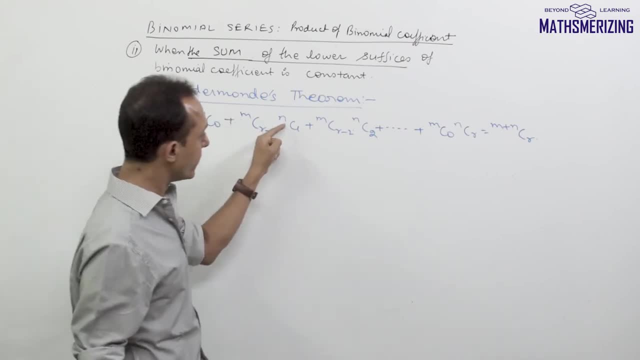 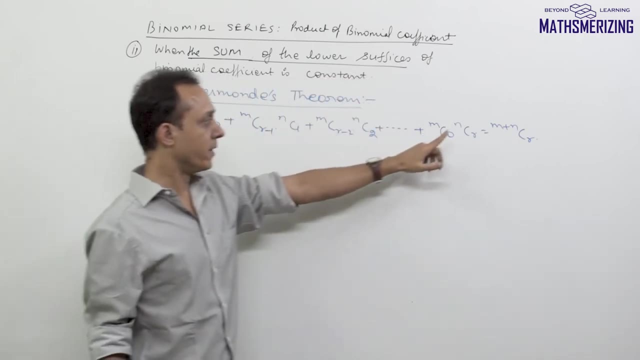 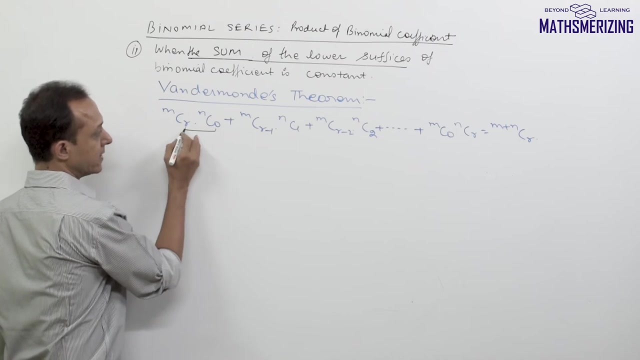 is mCr into nC0, mCr-1 into nC1, mCr-2 into nC2, mC0 into nCr, and we have to prove that it is equal to m plus nCr. Now, in this case, when I look at the sum of suffix, it is R. 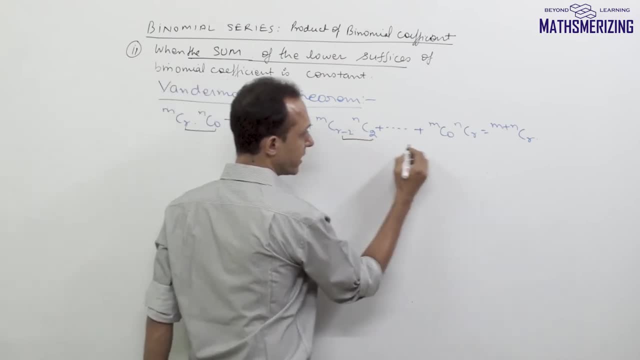 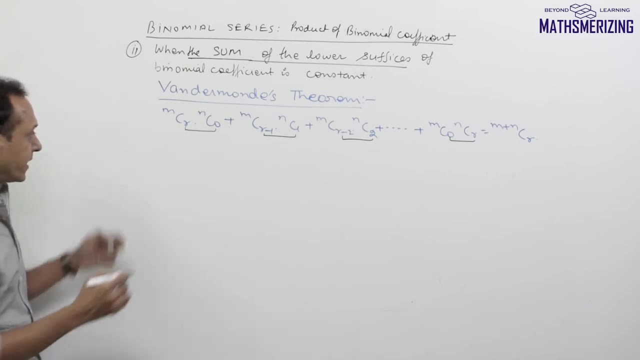 again R-1 plus 1 is R, R-2 plus 2 is again R, and then 0 plus R is again R. So that is sum of suffix. The sum of lower suffix of binomial coefficients is constant, So I will write the expression. 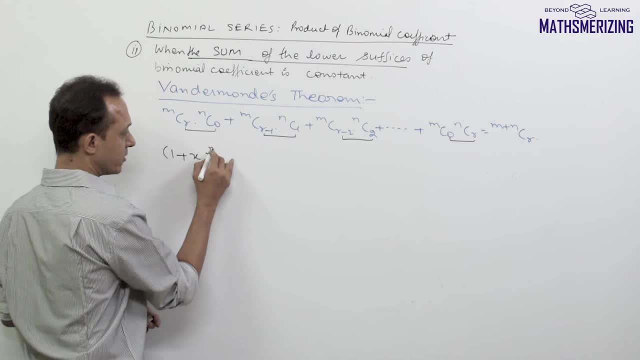 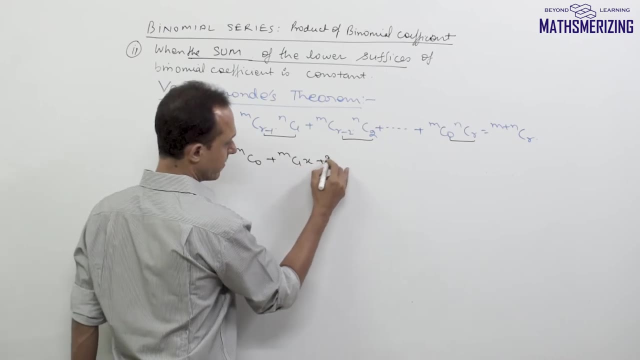 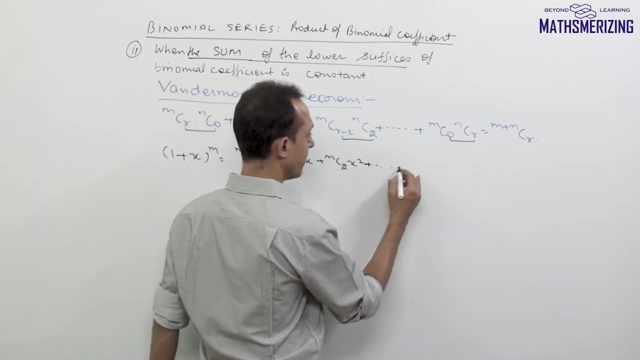 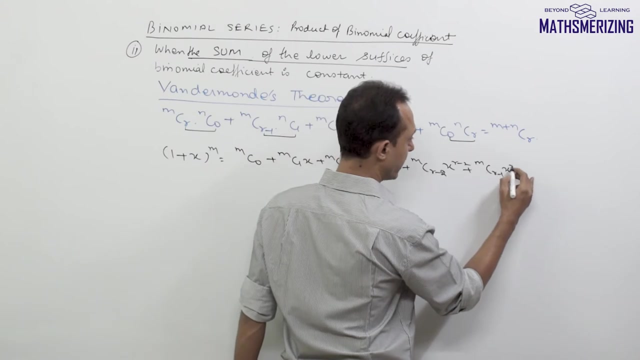 of 1 plus x to the power m, so it is mC0, mC1x, mC2x, square, and because I need mCr and mCr-1 and mCr-2, so I will write plus mCr-2 into x to the power, R-2, mCr-1, x to the power. 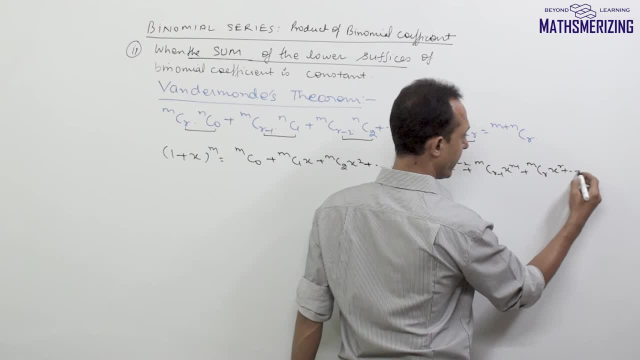 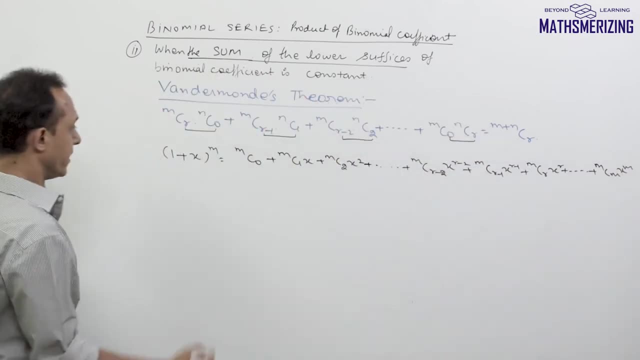 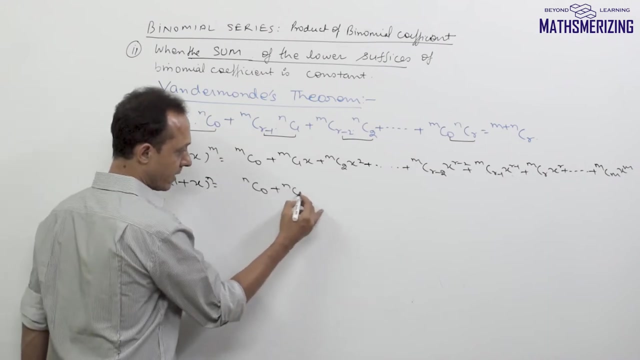 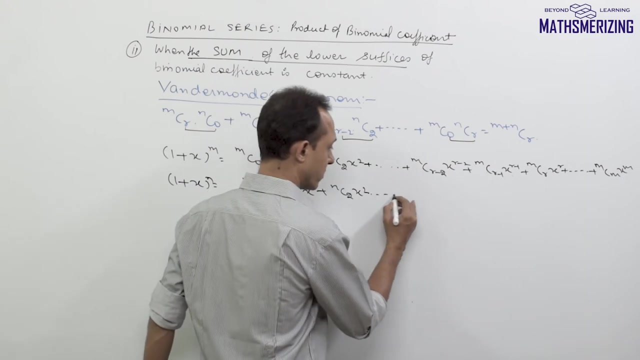 r, and then all these terms will continue up to mCm, into x to the power m. Now I will also consider the sum of this series, which is 1 plus x to the power n. So in this case it will be nC0, mC1x, mC2x, square. Now I need to multiply it till nCr, So it will be nCr-1. 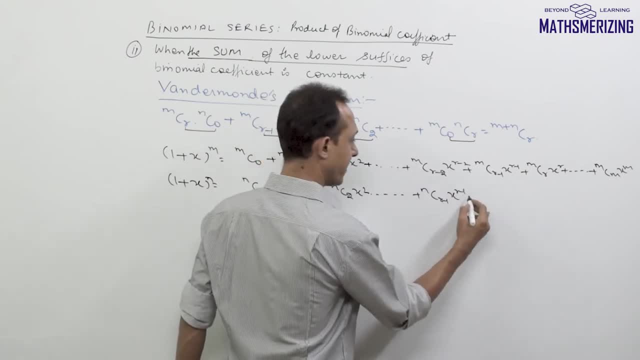 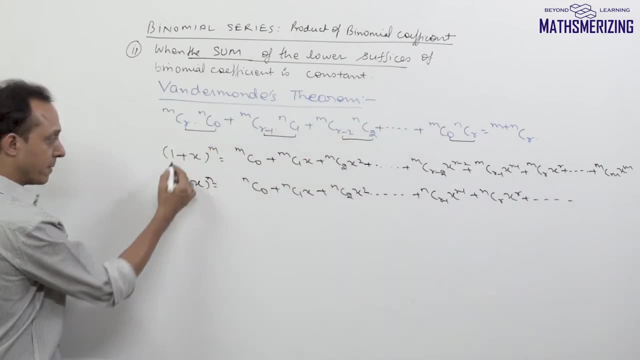 into nCr-2.. x to the power R-1 and then will be nCr into x to the power R. Now I will start multiplying them. So if I will multiply them then I will get 1 plus x to the power n plus n, and here 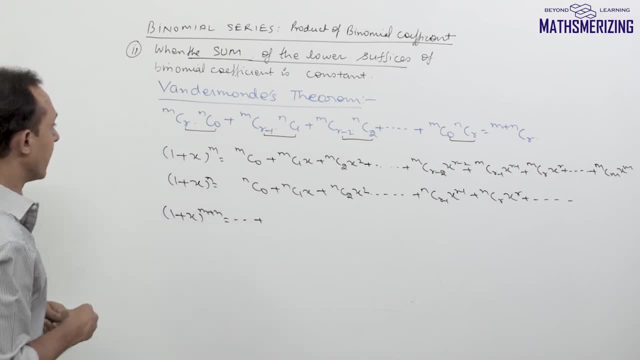 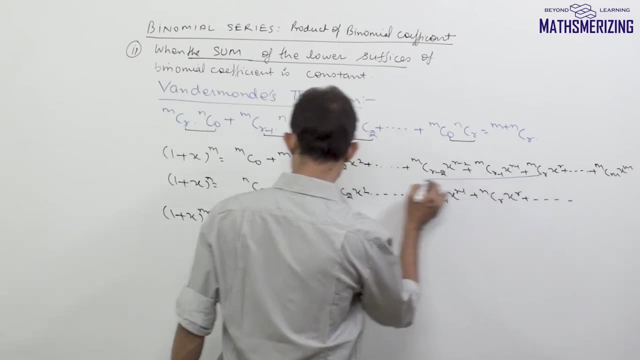 on the right hand side. I will ignore all other terms, So I will go for what I need. So what do I need? I need mCr to multiply with nC0.. So when I will multiply mCr with nC0, so I will get mCr-1 into nCr-2. 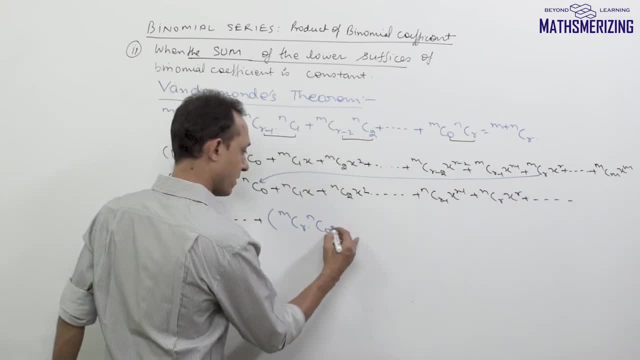 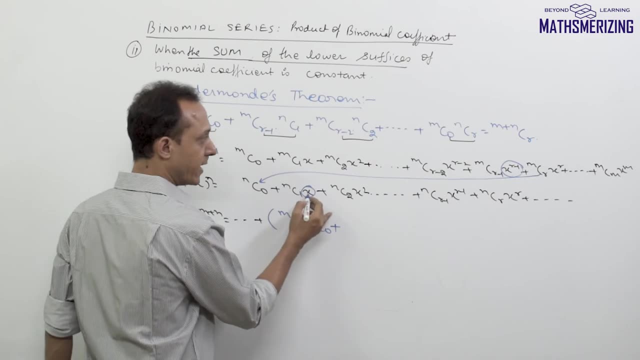 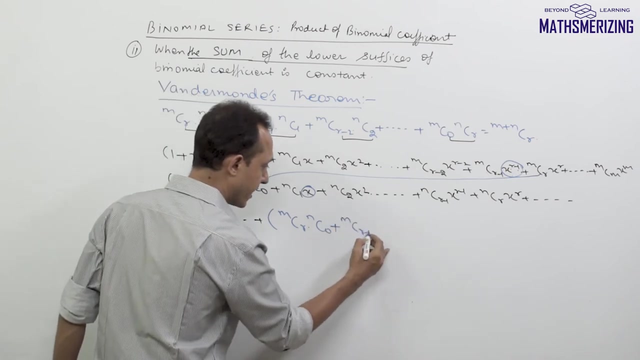 and it will be the coefficient of x to the power r. Now the next one is mcr-1 and nc1,, so mcr-1 and nc1,, so it is x to the power r-1, and this is x to the power 1, which again is x to the power r. so this is mcr-1 into nc1, so the 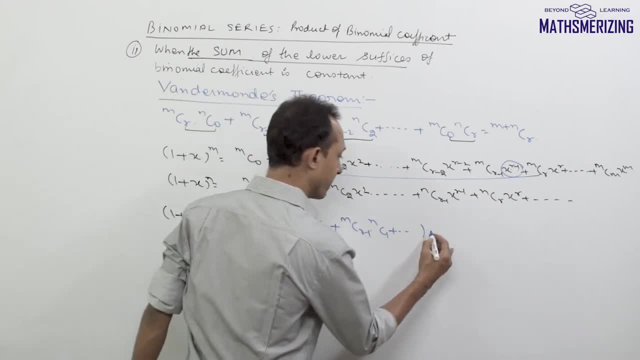 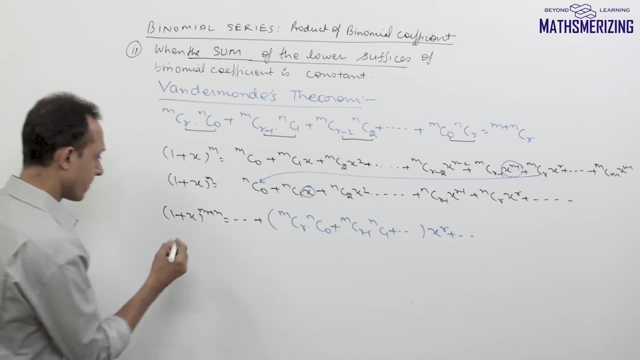 series that I need. so this series, it is nothing, but it is coefficient of x to the power r. So if I have to find the sum of the series, all I need to do is I just need to find coefficient of x to the power r from this left hand side. 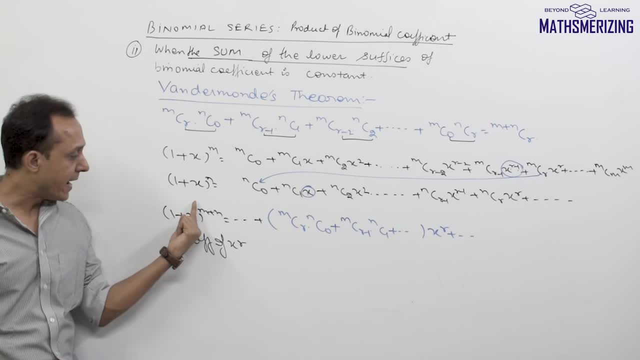 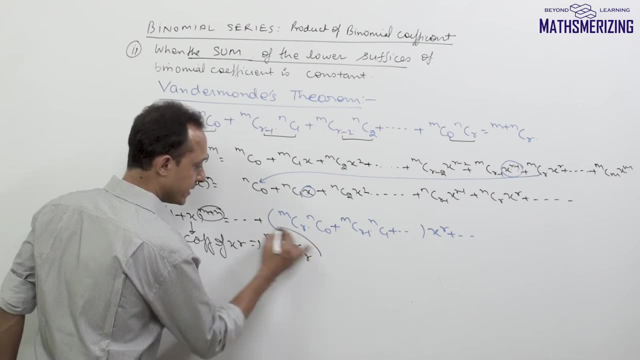 So what is the coefficient of x to the power r in 1 plus x to the power n? It is simply ncr, so n in this case is m plus n. so the coefficient of x to the power r simply will be m plus ncr, and that is your result, which is m plus ncr. 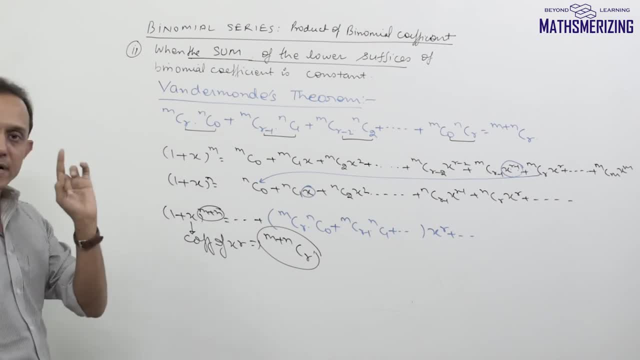 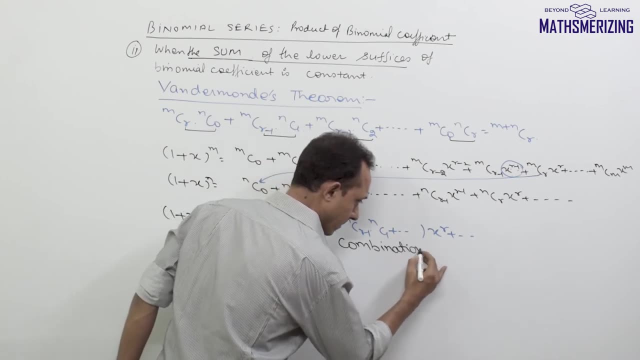 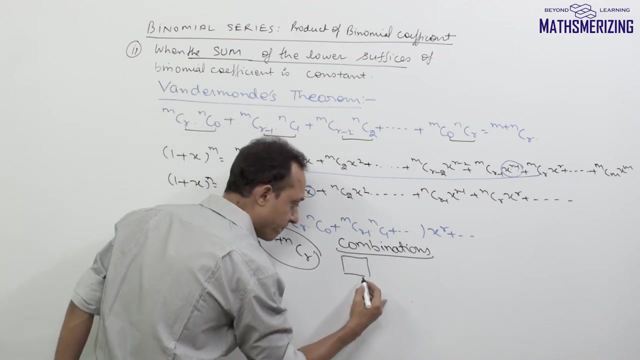 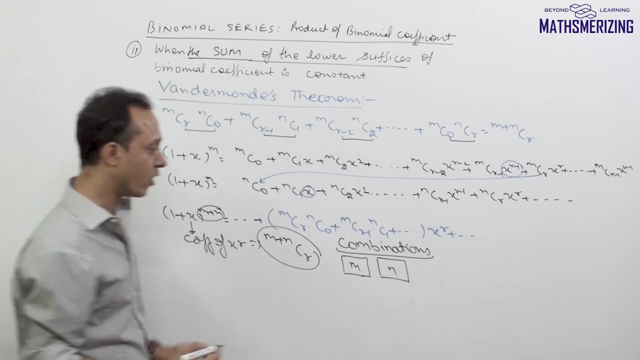 Now there is another way of solving this question And which is using combinational argument. Now suppose I have two separate group of distinct objects. So in first group let there be m objects and in second group let there be n objects. So we have altogether m plus n distinct objects. 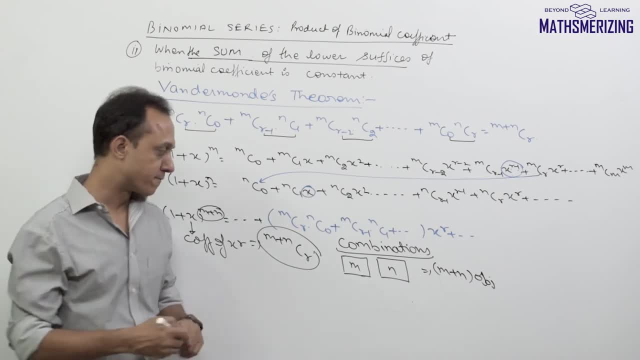 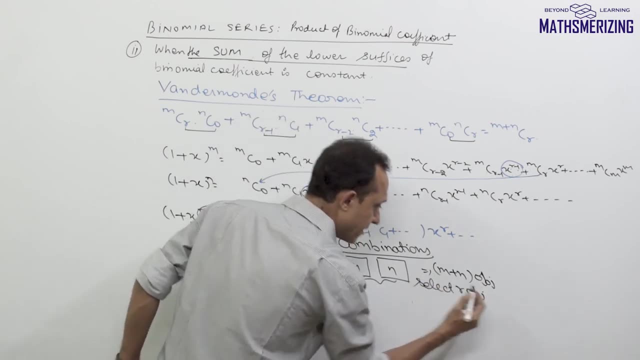 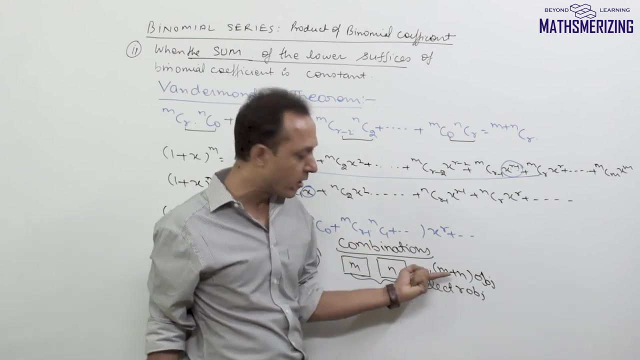 Now I have to select r objects from these m plus n objects. so I have to select r objects from these m plus n distinct objects. Now, in how many ways can it be done? So we clearly know that if I have to select r objects from n objects, it can be done in. 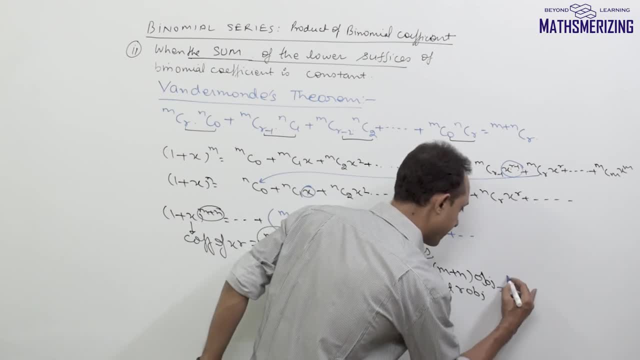 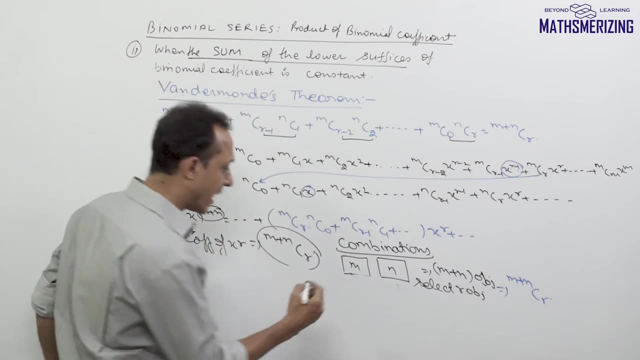 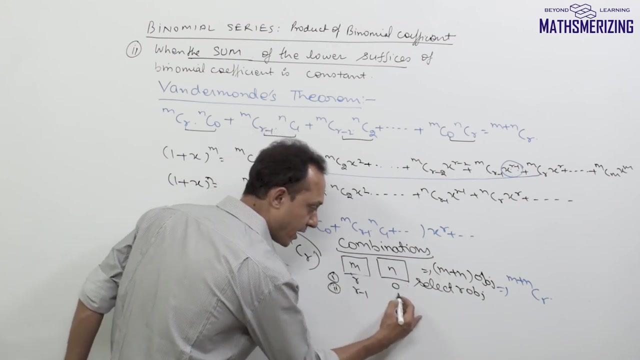 ncrt ways. So if I have to select r objects, then it can be done in m plus ncr ways. Now, another way of doing it can be If I have to select r objects from m and 0 objects from n, or I may select r minus 1 from m and 1 from n. it